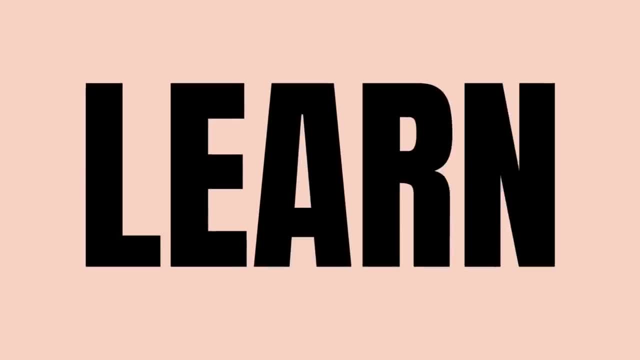 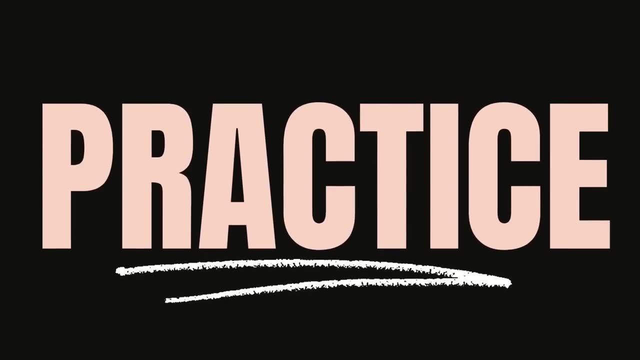 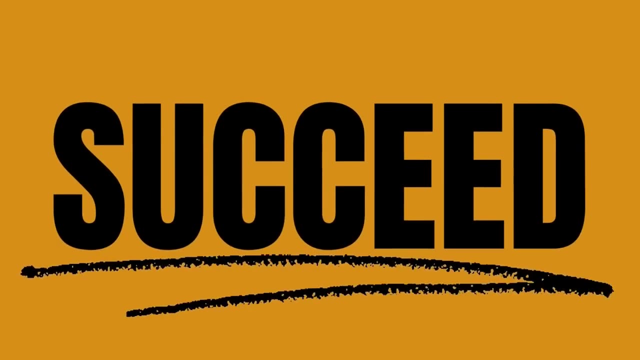 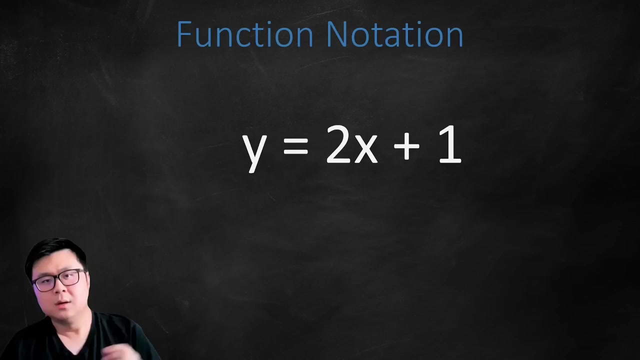 You got this. Come on, let's have some fun. Let's go. The first of the five is function notation, and in my opinion it's the most important too. Let's start with this function here. X is known as the input or the independent variable. 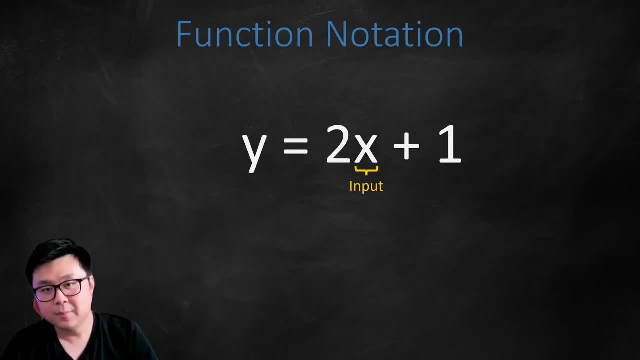 We get to select whatever number we want and replace X with a number, and it will undergo some type of algorithm here, As you can see, it will get multiplied by the two and then added to a one, and whatever answer we get after that is known as the output. Well, since Y is equal to 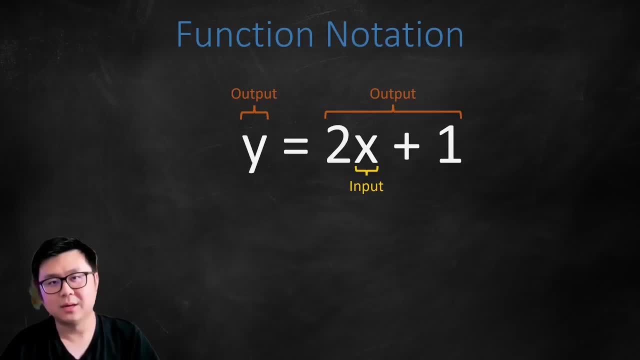 that entire right side. that means Y has to equal to the output as well, So Y is known as the dependent variable or the output. That is the basic premise of how a function works. As you probably know, we can rewrite the Y as F of X. That means F of X is also going to be the 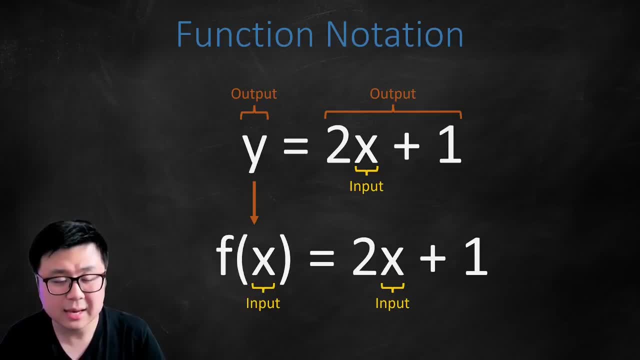 output. Nothing else changes here. X is still the input. and now notice X is also on the left side in a bracket. What does the F mean? Well, the F is just the name of the function and it doesn't have to be F. It could be any letter in the alphabet. F of X really means function of X. 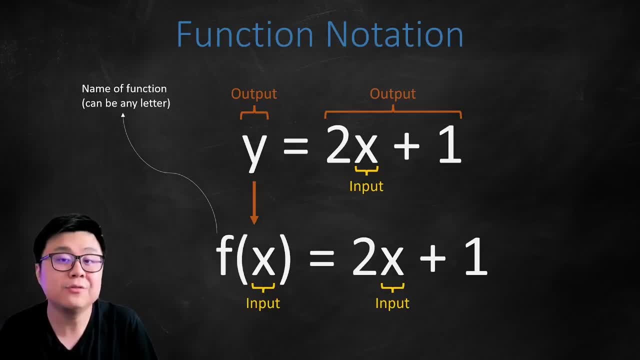 which actually means the result or the output, if you were to choose X as your input. So if I had F of 2 in the brackets, that means it will be the result or the output if you were to choose 2 as your input instead of X. F of X, we said, is the same as Y, and since Y is the output, F of X is. 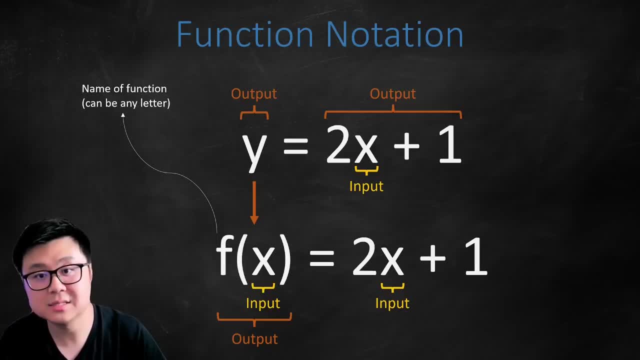 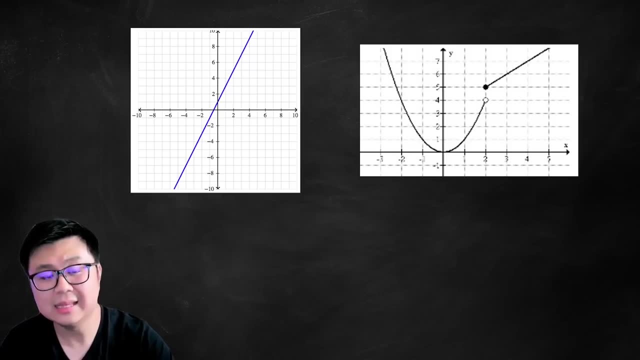 also the output, and we haven't changed a single thing on the right-hand side, so that remains an output as well. Let's take a look at the function on the left first. As you can see, it's clearly a linear function, something that you've probably learned before if you're taking calculus In a 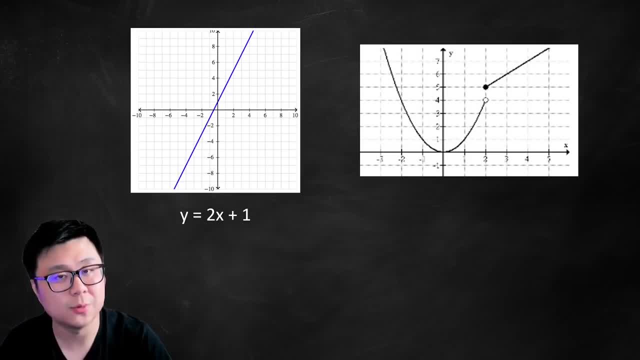 linear function. the equation for this one is Y equals 2X. So if you're taking calculus, you're going to have Y equals 2X plus 1.. Now we can also write it as F of X equals 2X plus 1.. Cool. 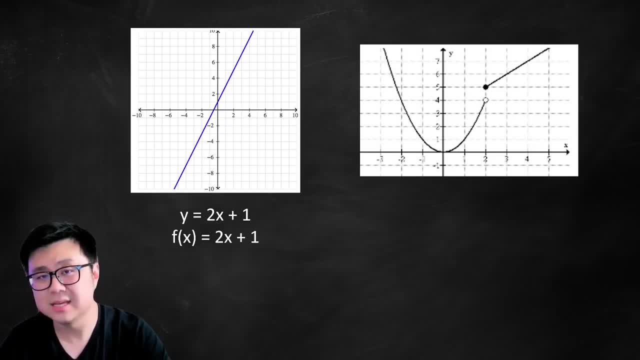 What about the function on the right? It's going to be pretty hard to represent this as one equation because there's no clear-cut pattern. This is called a piecewise function and we're not going to get into how to actually figure out the equation for this function. but what I want to 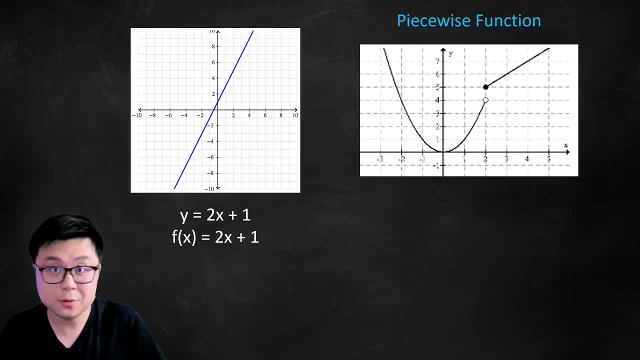 tell you is: if you see a function that you don't know the name of or that you don't know how to represent as an equation, you can always just call it: Y equals F of X, Even if you know the name of the left. we know this is a linear function. We know the equation. There's nothing wrong with. 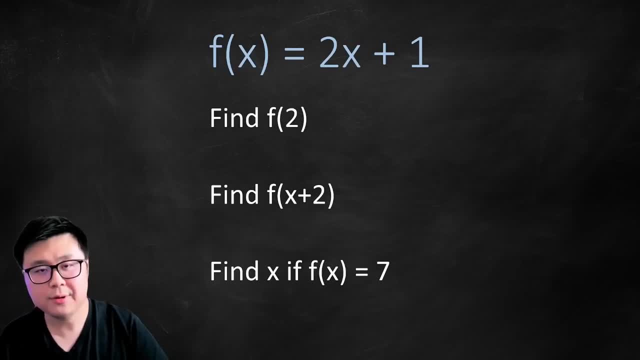 calling this, Y equals F of X as well. Now what if they were to ask you to find F of 2?? That means they want to know the output or the result if your input is 2.. So we're going to just write. 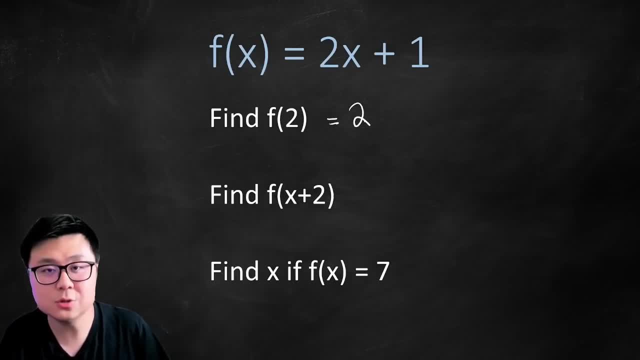 down, the equation equals 2,, but where the X used to be, because that's the default input. now we know the specific input is 2,, so we'll replace it in brackets with our 2 plus 1.. And then, to solve this, that becomes a 5.. So the output when your input is 2, is 5.. Your inputs don't even have. 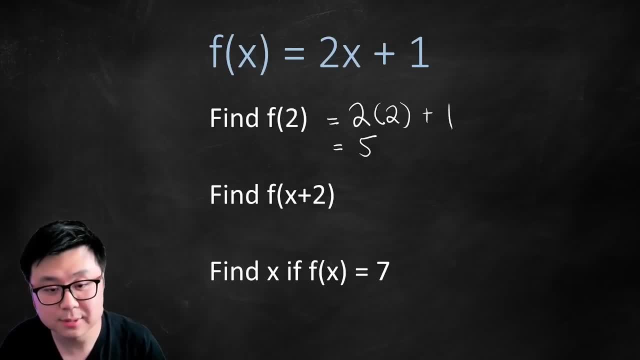 to be just numbers. It could be variables and numbers like the next one: X plus 2.. Nothing changes here. All we're going to do is we're going to replace our default input of X up here in brackets with our new specific input of X plus 2.. And don't forget that plus 1,. 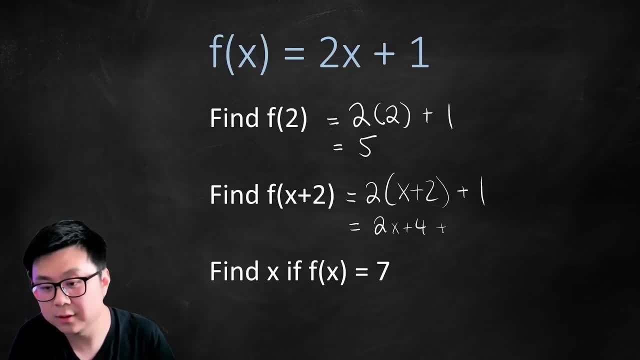 and then we simplify it and that becomes 2X plus 4 plus 1, and that gives us 2X plus 5.. Now the third example is the opposite. We're looking for X or the input, when we know the. 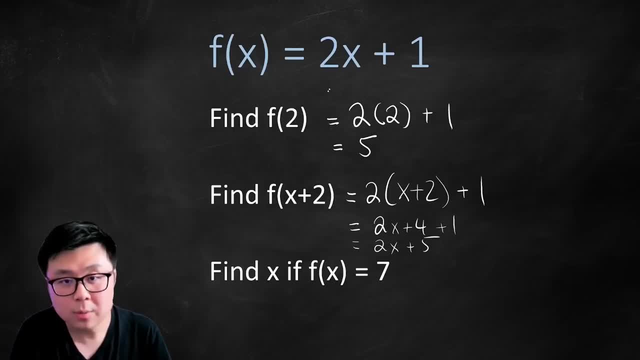 F of X or the output is 7.. So I'm not going to replace the X with my 7 here, because 7 is the output. I'm going to replace the entire F of X with 7.. So the equation becomes: 7 is equal to. 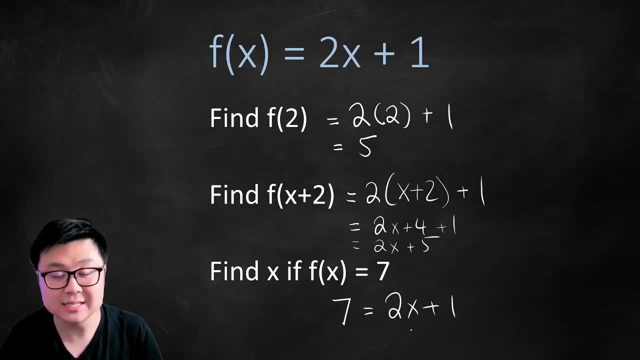 2X plus 1.. Notice, I left the X as it is because we don't know what X is, We don't know the input, And then we just do a quick algebra to solve Subtract 1 to get 6 equals 2X. 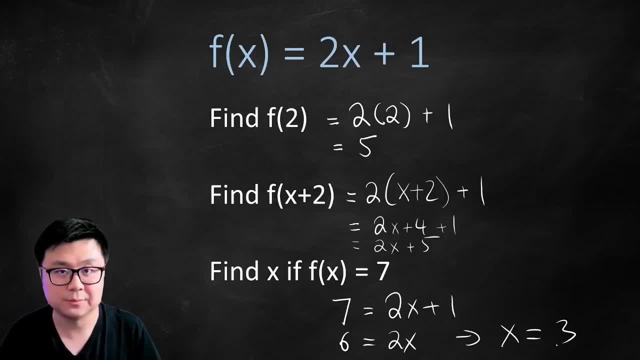 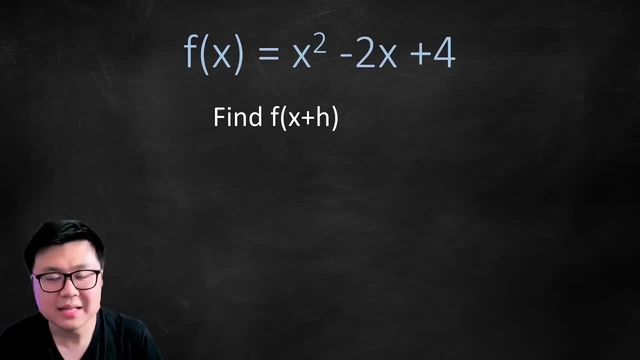 and then we ultimately get X equals 3 as our answer. This one might look weird because our specific input that they want, which is X plus H, has no numbers in it. But that's fine, We're going to just stick with what we know. We're going to replace our default inputs of X. 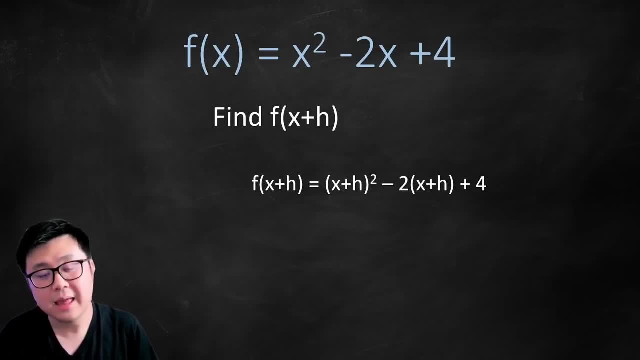 with X plus H. So it should look something like this, And then, with a little bit of simplification, foiling, expanding the brackets, it will look like this: Another application of function notation is to represent coordinates of a point on a function. 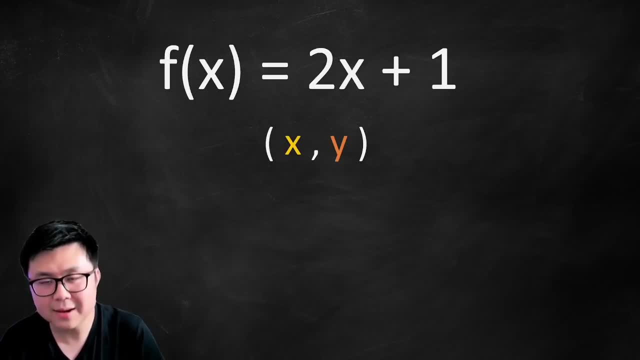 So let's take this function. We can say that there will be a random point with a coordinate X, comma Y that's located on this function. Absolutely, But didn't we say that both Y and F of X are outputs and they're the same? So we can also say that the coordinates of this point 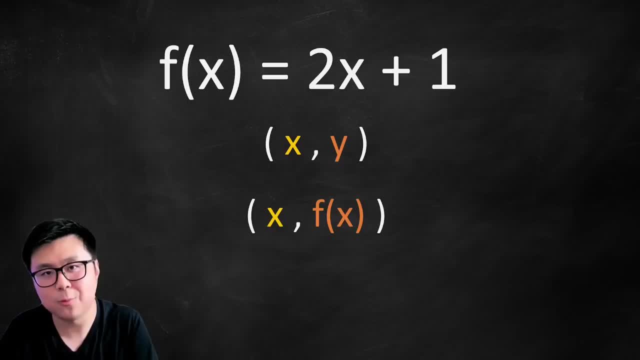 is X comma, F of X. Notice: we replaced the Y value of the coordinate with F of X. Let's take it one step further. Did we not have on the board here: F of X is equal to 2X plus 1? Well, if they're equal, then I can replace the F of X with 2X plus 1.. And that's also a way to. 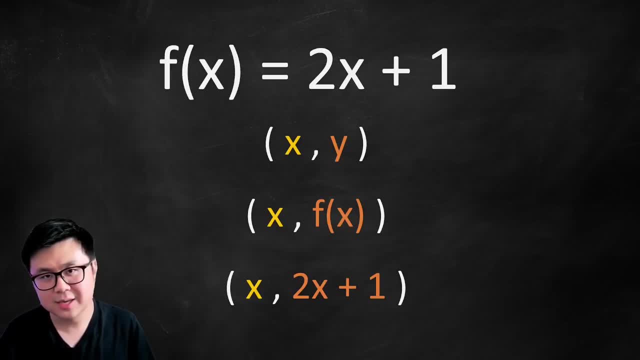 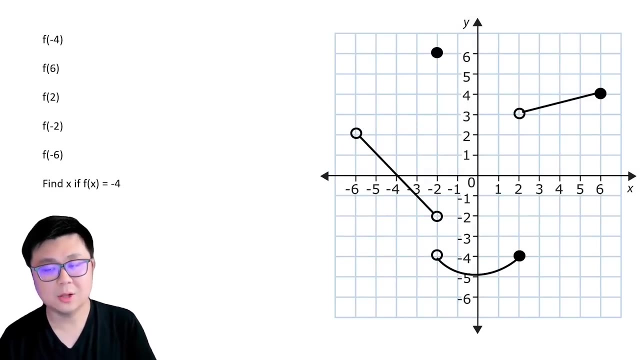 represent the Y coordinate of our point. So, as you can see, these three ways here are different ways to represent any random point on our function. You also need to know how to find inputs or outputs graphically, not just algebraically by plugging in. Let's take a look at this graph and look at: 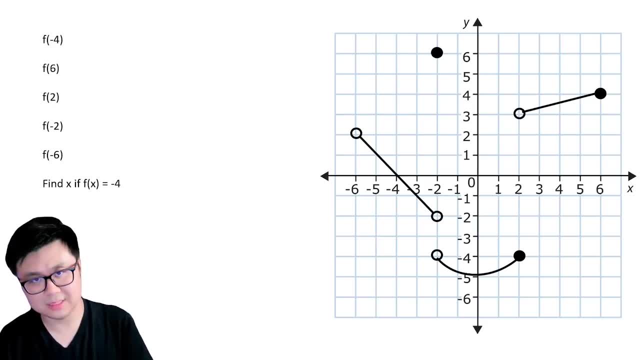 the first question. They're asking for F of negative 4, meaning when the input or the X value is negative 4,, what is the Y value or what is the output? So just scan the graph, Look for where the X value is negative 4, right here. And where is that point? Well, the Y value of that point is 0,. 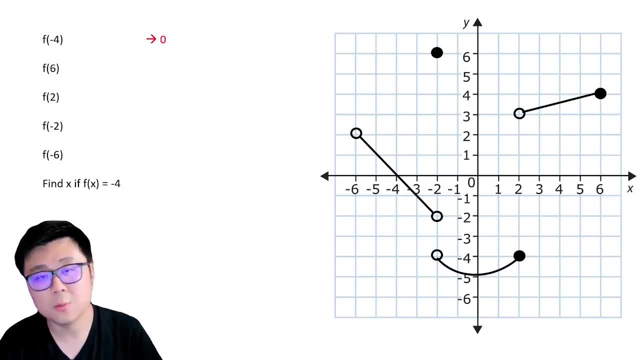 so the output is 0.. Same thing: F of 6.. When X is 6, what's the Y value? It's 4.. F of 2.. Well, when X is 2, notice that there is a circle above it and a dot below it. Remember an open circle. 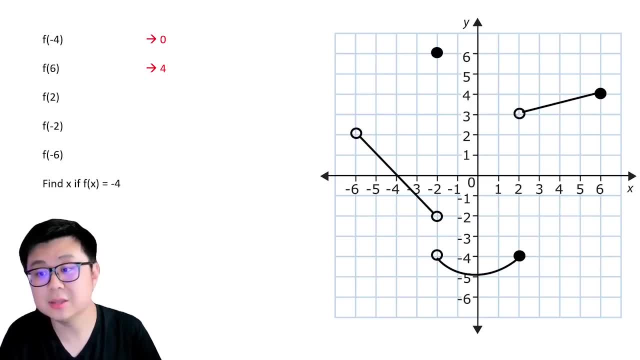 in math represents nothing. It represents a non-inclusive. so there's actually no point there. It's hollow. But luckily there is a point down here. so when the input or the X value is 2, the output is negative 4 for your Y value, Next F of negative 2.. When your input's negative 2, notice there's. 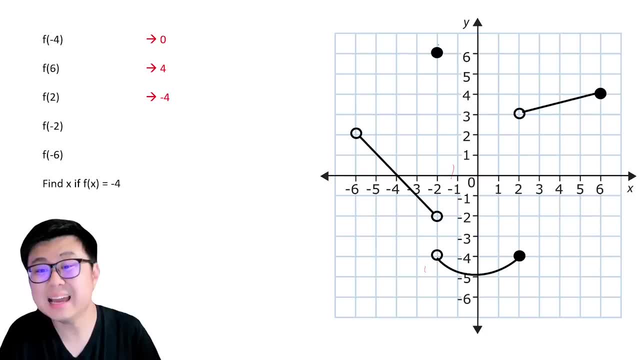 two empty circles here. There's nothing there, but luckily up here there is a random dot where X is negative 2 and the Y value is 6, we'll take that The Y value or the output is 6.. Next, f of negative 6.. This time do you see anything along the line of x equals negative 6 aside? 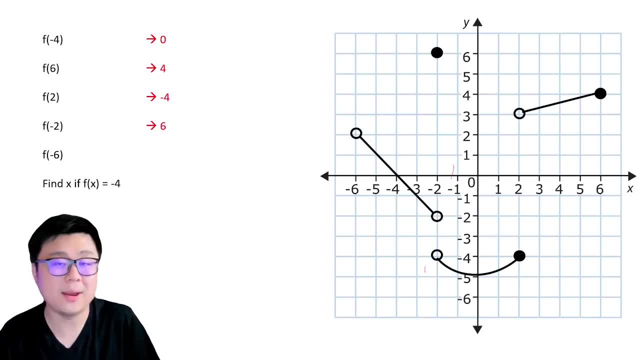 from this empty circle. No, which means there's no point. there's no y values at all when your x value is negative 6, so we put d and e or does not exist. Lastly, they're asking for x when your f of x is negative 4.. That means this time they're giving you the y value. 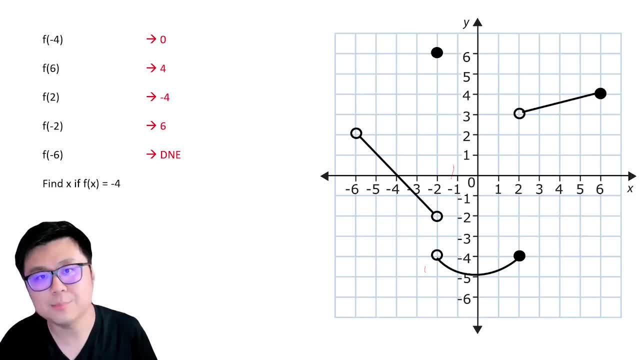 or the output is negative 4, they're asking for the x or input value. So let's scan up and down this time for a y value of negative 4,. as you can see, it's down here and there is an open circle to the left- very useless, but luckily there is a closed circle to the. 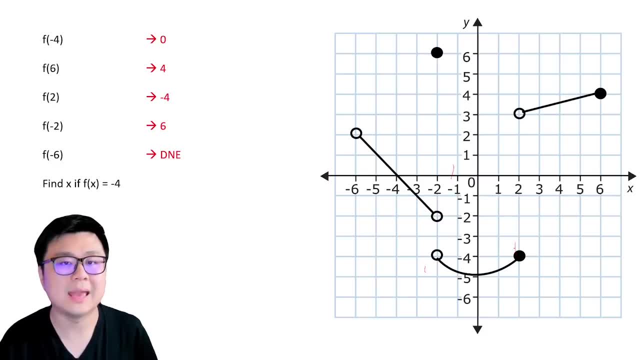 right, and the x value is 2, so the answer is 2.. Lastly, let's see how we can represent some of these as coordinates of a point. So the very first question here: f of negative 4, we know that the x value is negative 4 and 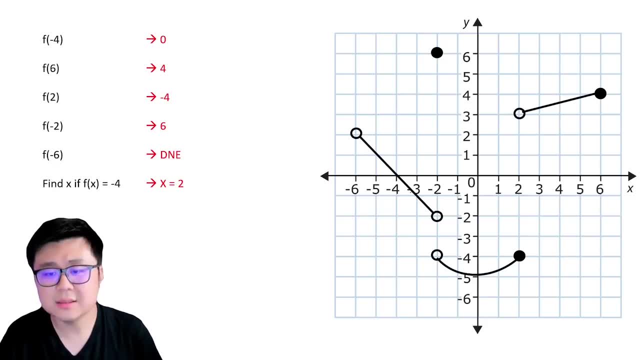 we just figured out, the y value is 0.. That means this point right here should have the coordinates negative 4 comma 0.. Yes, but we can do this a different way as well. Our input, or x value, is negative 4,. okay, Then our y value. we can represent it as f of x, remember, but not. 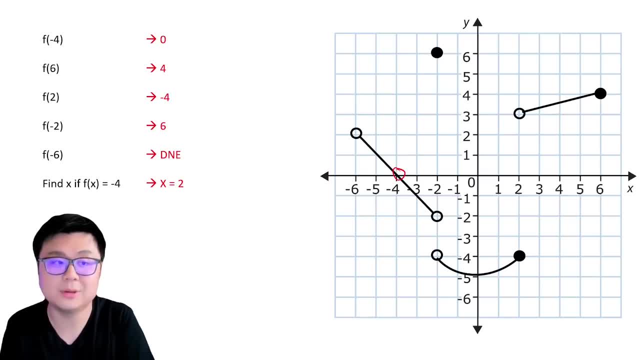 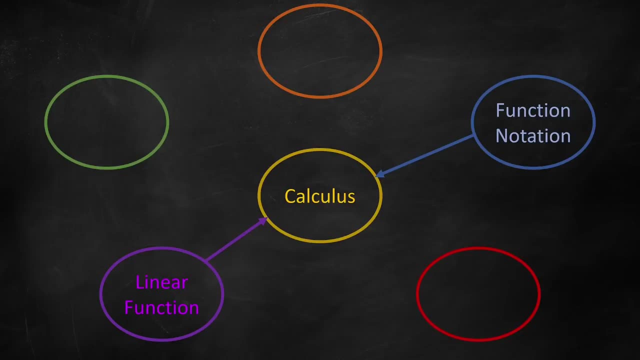 f of x, because our input is no longer the default x. our input is, specifically this time, negative 4.. So the point can be represented as negative 4, comma f of negative 4.. The second important concept is linear functions. The third important concept is: you don't have to know the entire chapter or everything. 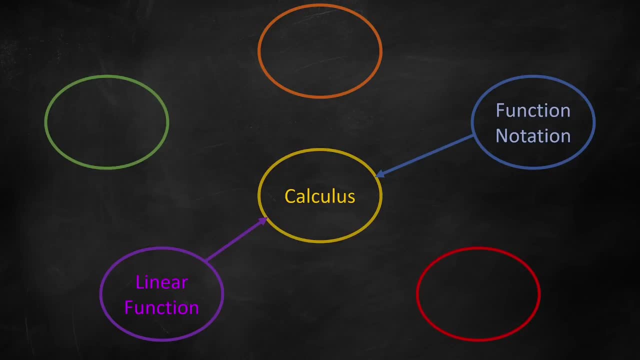 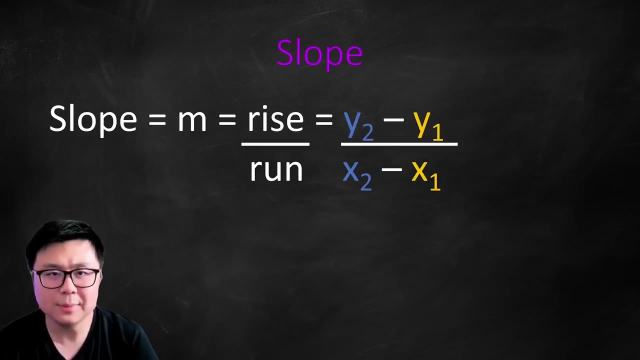 about linear functions. There's only two main things you've got to refresh your mind of when it comes to linear functions before you start calculus. The first thing we're going to talk about in linear functions is slope. Well, slope is represented by the letter m and it's calculated with rise over run, but a much more useful 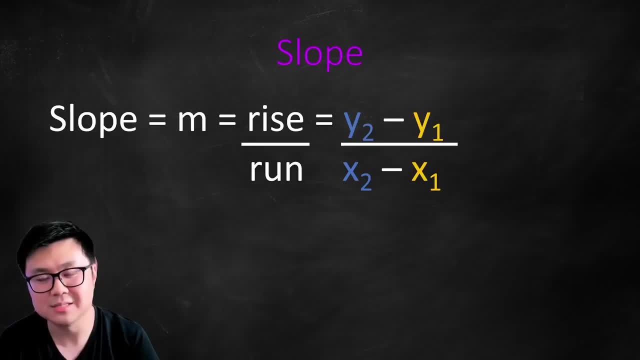 equation to calculate slope is y2 minus y1 over x2 minus x1, given that you know two separate points on the graph, Denoted as x1 and y1.. y1 for your first point and x2 and y2 for your second point. Let's take a look at this function. 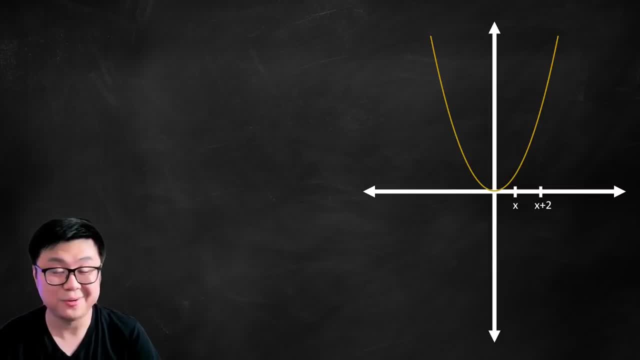 on the screen. Some of you might be thinking this is a quadratic function or a parabola, and you're probably right, but we're going to be lazy here and we're going to call this: y equals f of x. Let's find a point on this graph, shall we? Let's say this point right there. Okay, what is its? x? 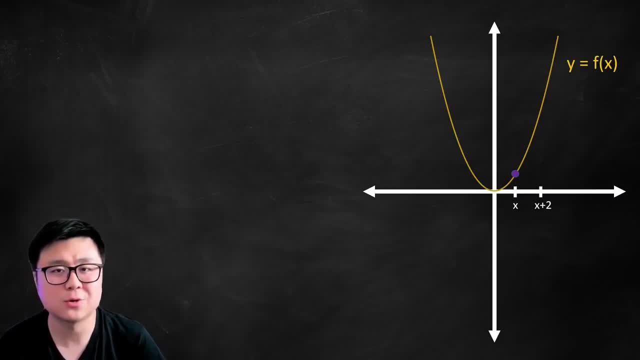 coordinate? We don't know, do we? So we're going to call the x coordinate x. If the x coordinate is x, then what about the y coordinate? Would the y coordinate be y? Sure, but you'll see later in calculus we don't like that. So what's another way we can represent the y coordinate? Remember? 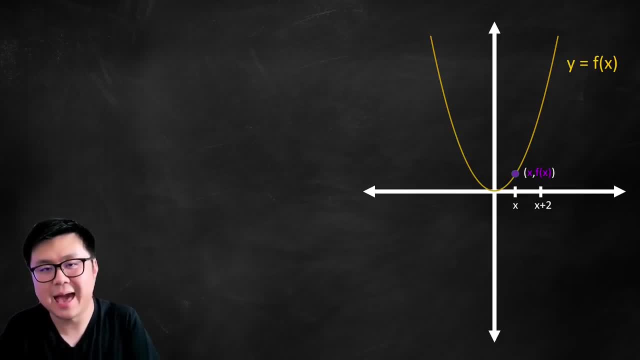 earlier. we can represent it as f of x. So the actual coordinates of this unknown point can be written as x, comma, f of x. Okay, let's do another point. Let's say up there: What is the x value of that point? I just hypothetically said x plus 2 because I have no idea what it is. So if the x 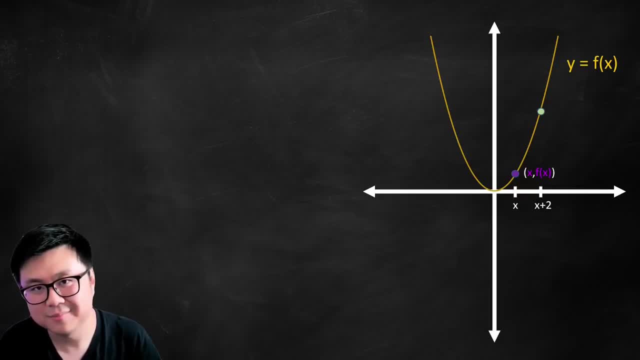 value is x plus 2, what is the x value of that point? I just hypothetically said x plus 2, because then what should the y value be? Ah, x plus 2, comma f of x plus 2.. So all of a sudden, now we have 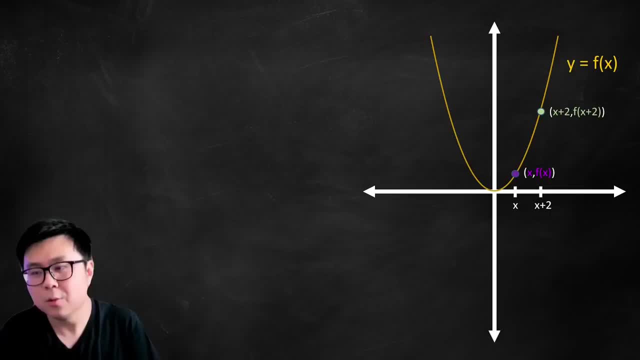 the full coordinates, although they're not actual numbers. but whatever, We have coordinates for both points, which means: can we now find the slope? Of course we can. If we have two points, we can plug it into our slope equation and find the slope. But let me ask you this: What slope are we? 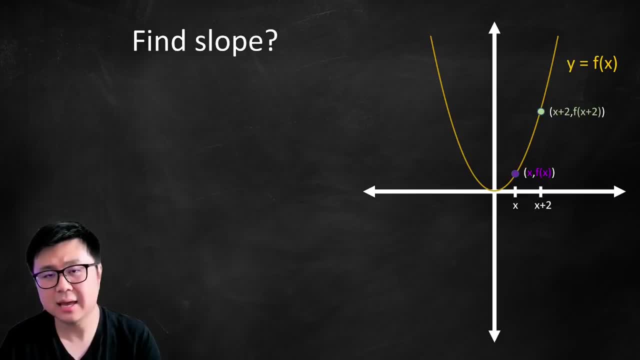 actually finding if we're using these two points. Constant slope only works for linear functions. This function is not linear, which means if we were to find a slope using these two points, we're actually finding the slope of an imaginary linear line that connects these two points, and that line is called the secant line. We're not going to go. 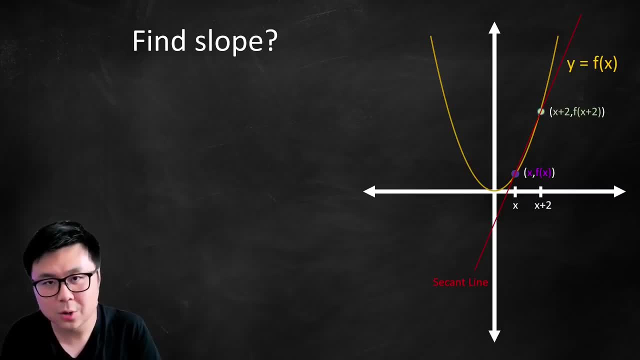 too much into this. You will learn this in calculus, but for now just know that when you're finding two points on a curved graph, that slope you're finding is not the slope of the curvature. The slope is just that of an imaginary linear line that connects the two points. Let's put these: 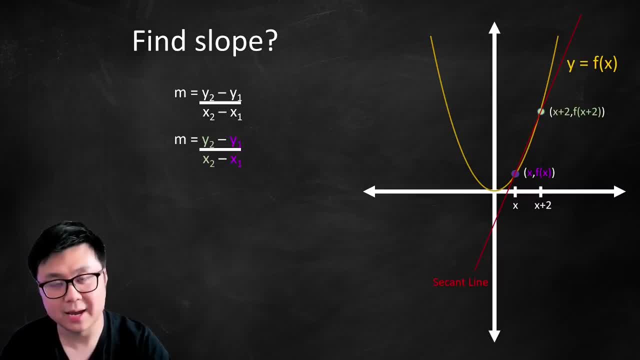 points into the slope equation. Be careful to label what's your x1, what's your y1 and all that, and once you plug it in, it should look something like this: We can simplify the bottom: The x is actually cancelled out, so our slope will look something like this. I know it's not a real. 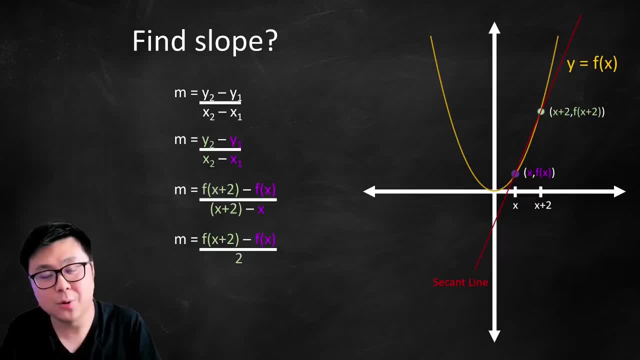 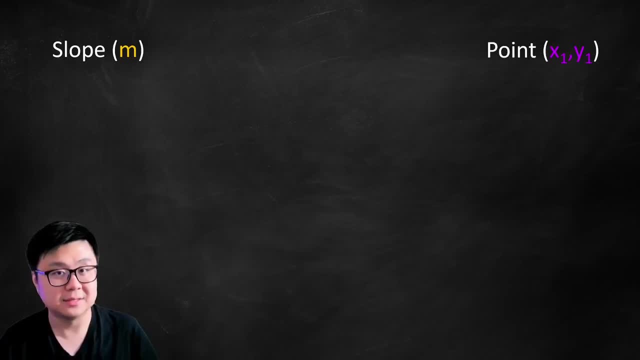 number. It's not an actual slope number, but as long as you know how to do this and why you're doing this, you should be fine for calculus. The second thing you got to know for linear functions is that you can take the slope, which is something you will find, as well as a point, something that 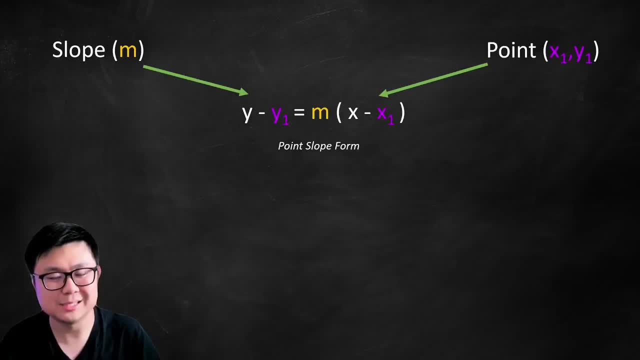 I'll probably give you and combine them into the point slope form, which should look familiar, and then from there you could turn it into the slope intercept form. y equals mx plus b, where the b is the y intercept. but it's not that important here. Some teachers are actually okay if you leave your. 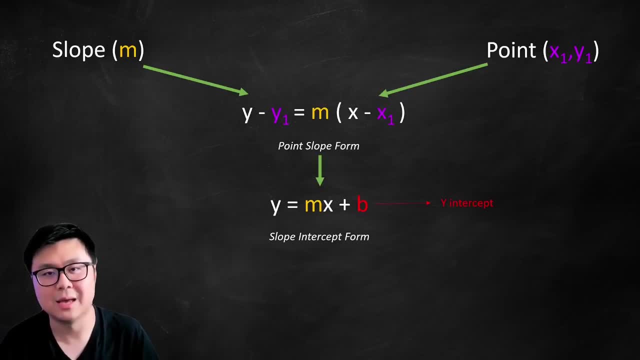 answer in the point slope form, so there's no need to go into. y equals mx plus b. You can also get it to the general or standard form, but honestly it's not that important. You can also get it to be in calculus. You will never need to do that, so don't worry about that form. The third concept: you 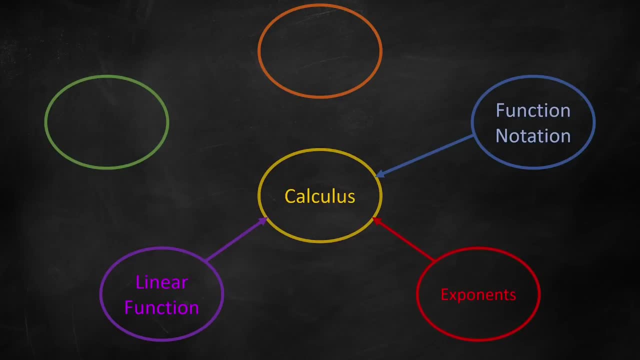 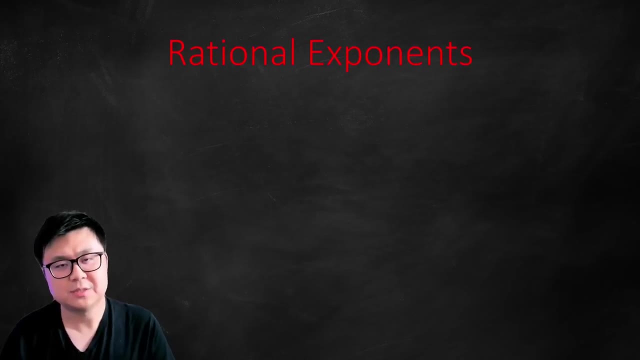 must be good with before starting calculus is exponents. Here I'm stressing on three specific rules or applications of exponents. Let's take a look. The first one is rational exponents. For example, if you were to have something like three to the power of three over four, that can be written. 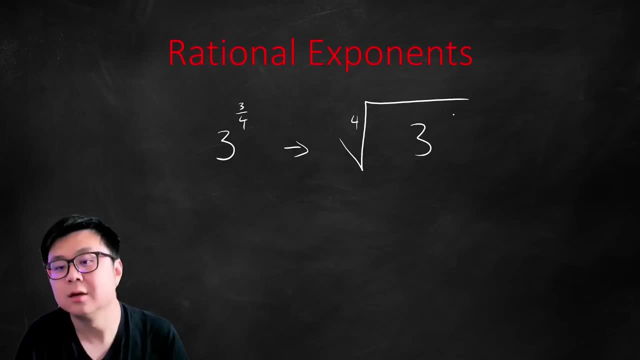 as the fourth root of three to the power of three, or you can write it as the fourth root of three and then all to the power of three. We can also go backwards. Maybe we have something like the square root of x to the power of three. We can write that as x to the power of three over. 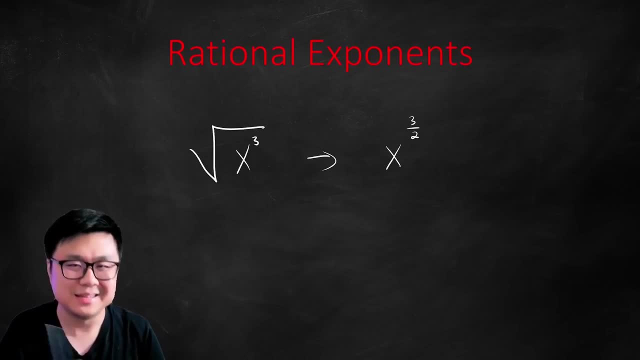 two. Going this way is way more important than the other way we just did. In calculus you have to be very, very comfortable going from a radical to a rational exponent. The second rule is negative exponent rule. Up until now you've probably used it mostly to get rid of negative exponents. 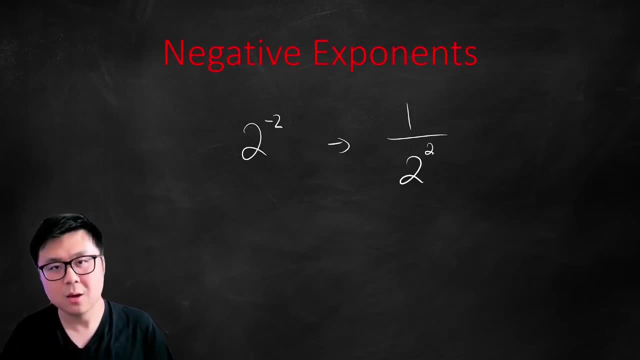 Well, in calculus that might happen, but for the most part you have to take something with a positive exponent and rewrite it as a negative exponent, just for the sake of getting rid of fractions. The last one's a bit funky here. In this case you have to be good at taking out the greatest common. 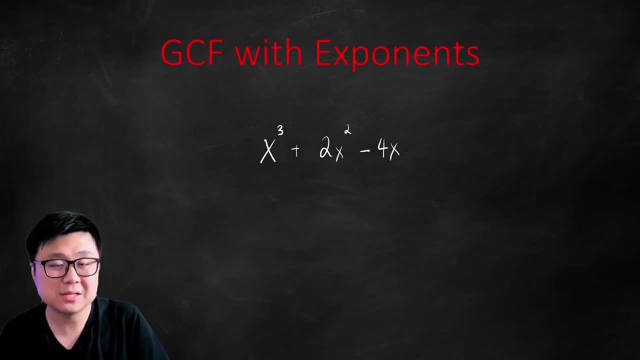 factors with exponents. Let me explain. Let's take a look at this expression here. Can we find a greatest common factor? and the answer is yes, They all share the same common factor. Let's take a look here: x to the power of one. Well, how do we factor out the greatest common factor? We divide all. 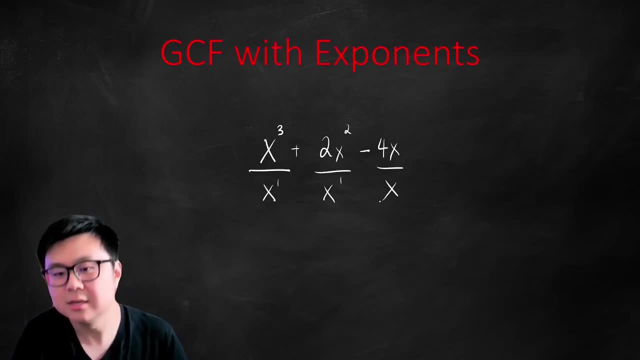 terms by x to the power of one or just x. and when you do that, we're using quotient rule, So we're subtracting, so you end up with x on the outside, because that's my greatest common factor, and on the inside, x cubed over, x is just going to be x squared plus 2x minus 4.. That's the GCF In this. 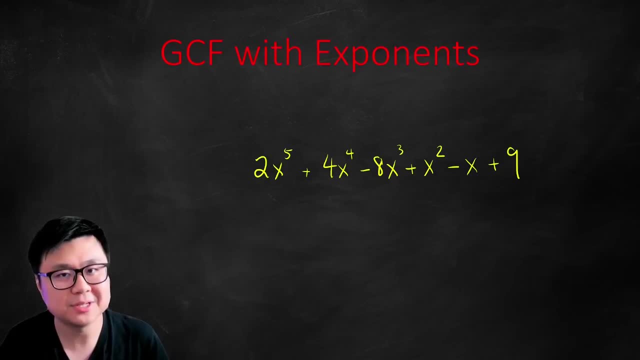 case, let's say they force you or you're forced to factor out an x to the power of one. So we're going to divide each term by x to the power of four. Well, you might be saying: not every term here has x to the power of four. Only the first two terms does, and then afterwards they don't have. 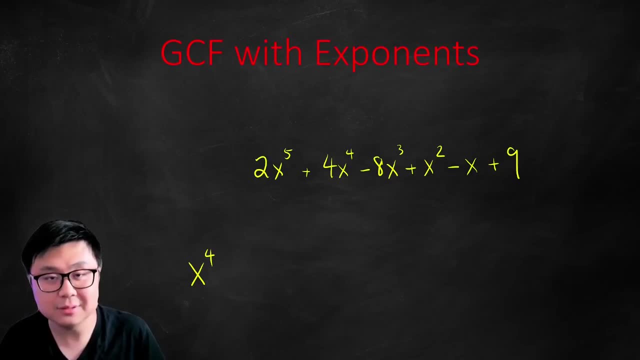 enough x's, It doesn't matter. You still have to factor out the x to the power of four, and it's possible if you just stick with the quotient rule. So let's see here: We're going to divide each term by x to the power of four, and when we do that we're going to subtract the exponents. and let's 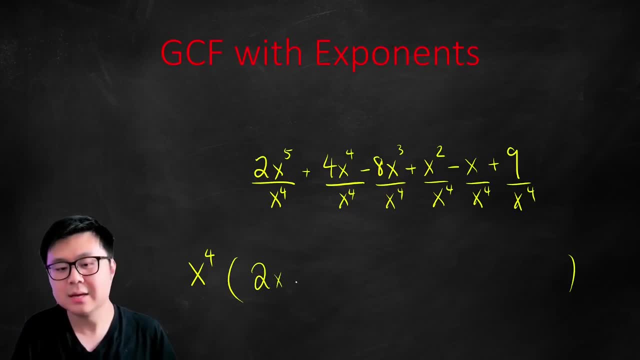 see what happens: The first term becomes 2x, The second term becomes 2x, The second term becomes four, and then, starting with the third term, we actually have more x's on the bottom than the top, so it becomes 8 over x plus. and then here we have two more x's on the bottom, so it'll be 1 over x. 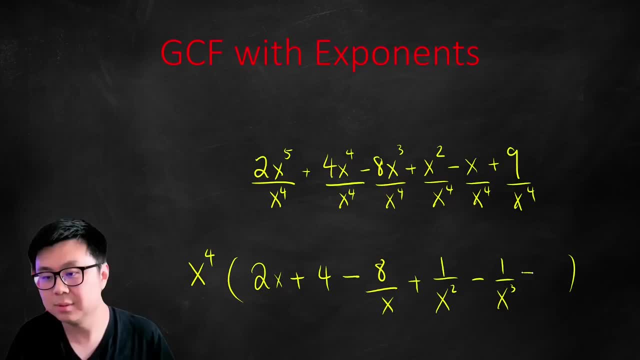 squared minus, 1 over x, cubed plus, and then we keep the last one, exactly the same, 9 over x to the power of four. That is what you have to do here. It might look weird, It might feel awkward, but you need to know how to do this for calculus. The fourth concept is domain inversion. 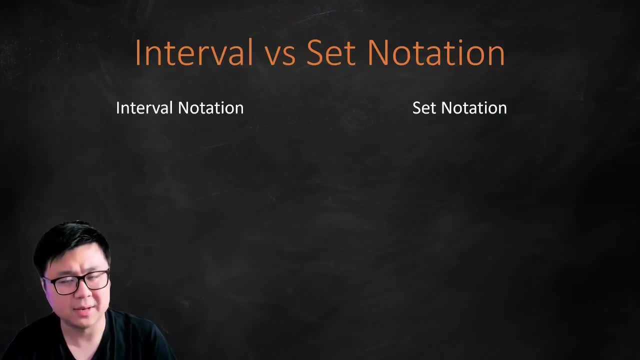 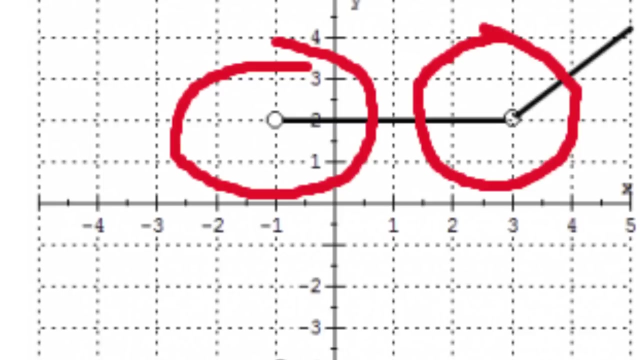 Range Recall. there's two different notations for writing a domain in range. There's interval notation and set notation. In the interval notation the brackets mean everything. A round or open bracket means that it's not inclusive, whereas a square bracket means it's inclusive, Non-inclusive. 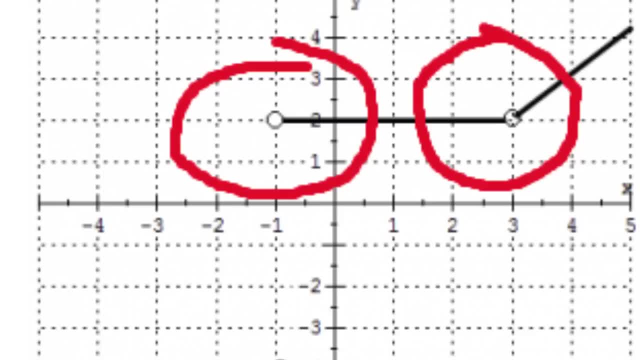 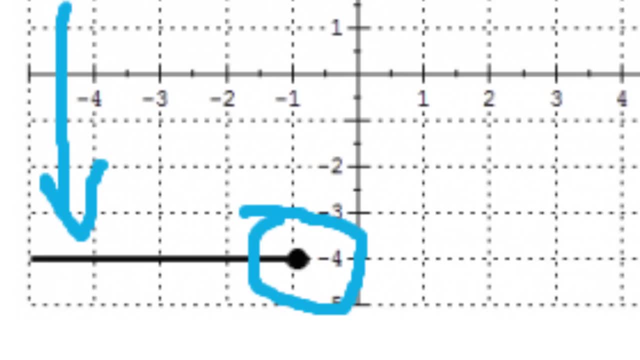 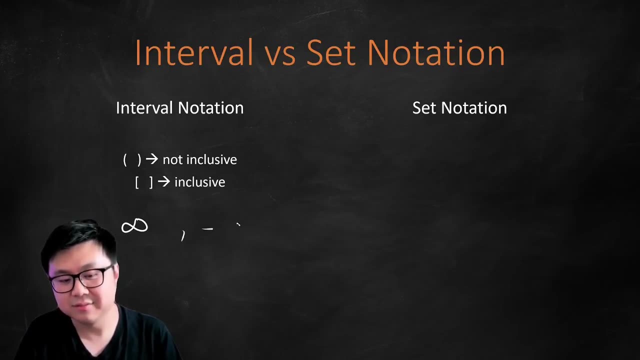 on a graph would be something that is like it's open circle. That means we don't have an actual point there, whereas inclusive means it's either the graph running right through or there's an actual filled in dot on the graph. In interval notation we also use the infinity sign for positive infinity as well as negative infinity. 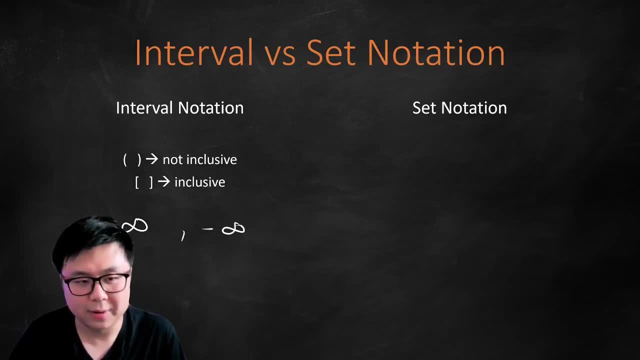 if we're going towards the left. So a typical domain or range in the interval notation could look something like an open bracket with a negative infinity, for example, and then it goes to like four and let's make it inclusive. Keep in mind, if you're going to use infinity or negative infinity, you 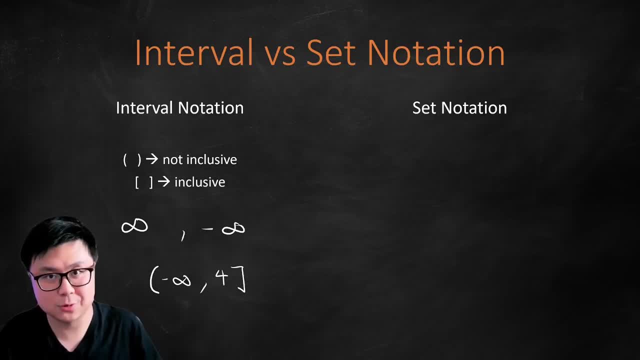 can't ever include infinity, because infinity literally means it keeps going on and on, so it should always be paired with an open bracket when it comes to infinity. That's something where you would use stuff like greater than or less than, or greater than or equal to, or less than or equal to, and you would usually set it up like with a bracket here. put x. 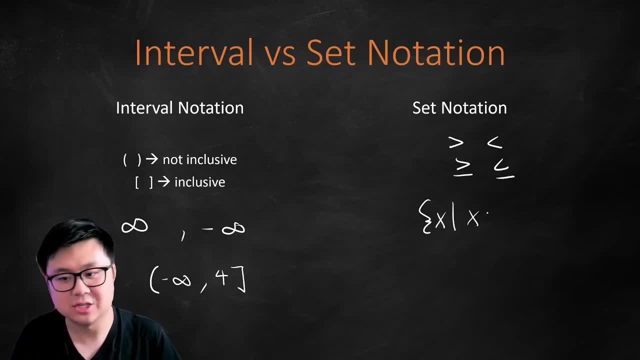 if you're doing domain with a vertical line, then you can say like x has to be greater than or equal to four comma x, er, and then close the bracket. Some teachers don't even care about the brackets. you can just write x has to be less than three or x er if you're doing domain, and then just replace. 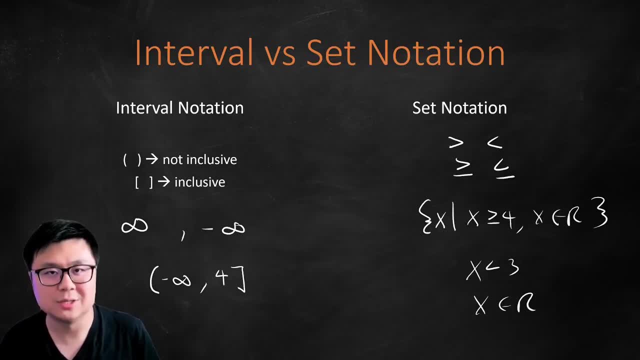 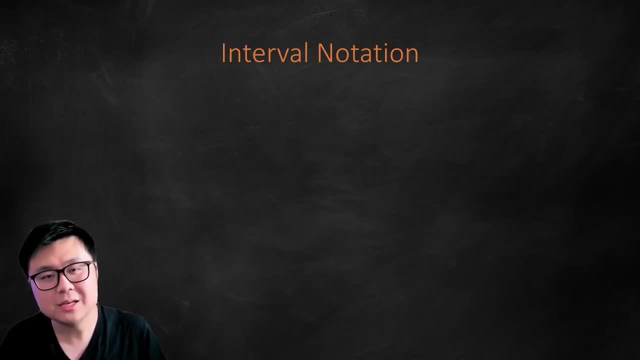 the x's with y's. if you're doing the range, That's set notation, But unfortunately in calculus you don't actually use too much of this. So, focusing on the interval notation, you're going to need to use this when you're doing something called curve sketching. 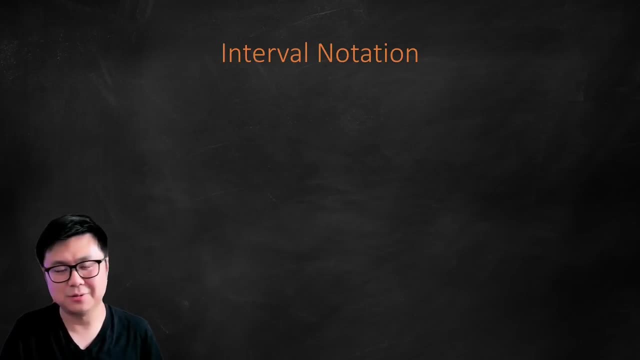 and they're going to ask you at which intervals is the graph increasing or decreasing, or concave up or concave down? So just know how to use interval notations. and then there's this thing: here There is a u and this stands for union. Now, before calculus, if you were to have two separate domains, 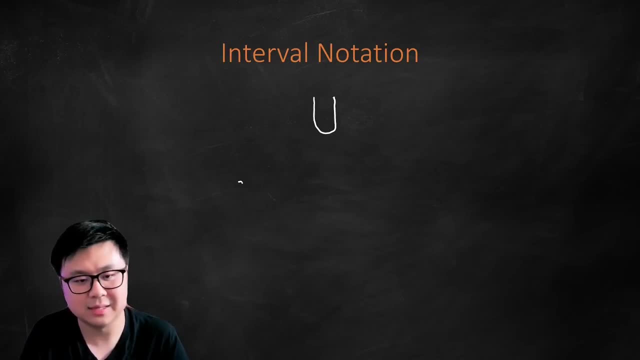 you would do something like this. You would say: it spans from, let's say, negative four to zero inclusive, and then you can write the word and. or. you can write or. it starts from positive two and it goes to positive ten inclusive, something like that, But instead of the word or, or, and you just 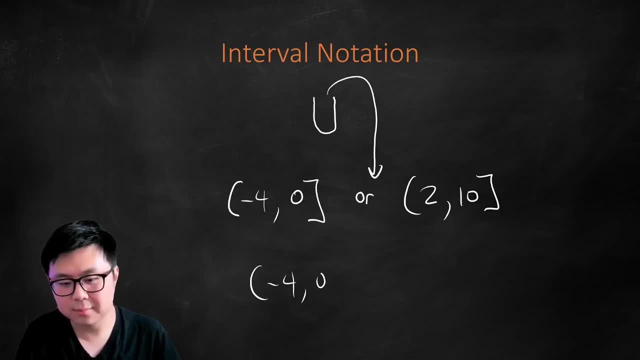 replace that with the? u, So it will look like negative. four comma zero, and then u for union and then two comma ten. Just keep in mind that's what the? u is U stands for. it just means and, or, or. Last but definitely not least, is the concept of composite. 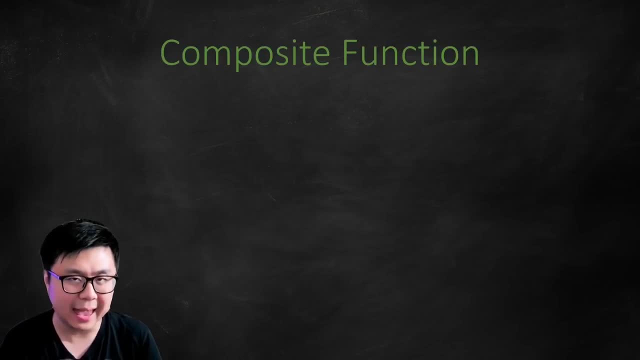 functions. A composite function is when you take the outputs of one function and you substitute it into the input of another function. Simply put, you're just going to take one entire function and shove it into where the x is in the other function. Let's take a look at our two functions. 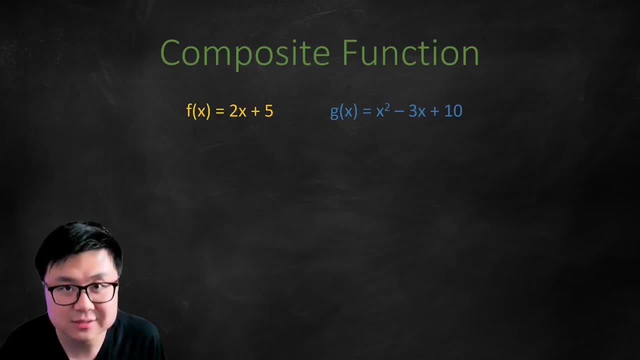 here We have an f of x function and we have a g of x function. If they're asking for f brackets, g of x: close brackets. notice the x used to be in the brackets for the f of x. It's not there anymore. is it The x or the input got replaced by the entirety? 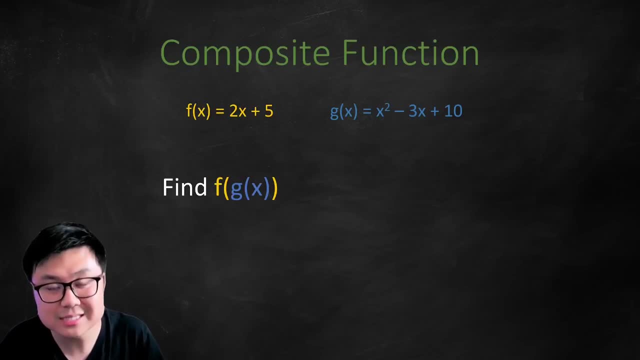 of g of x, which is the output of your g of x function, isn't it? So we're taking the output of g of x, or the entirety of g of x, and we're placing it where the x used to be in our f of x. 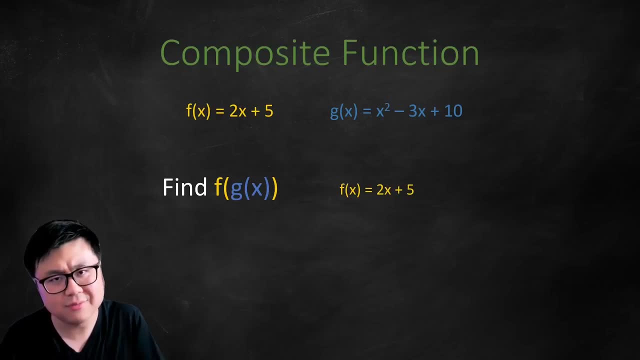 function. How do we actually do this? Well, we're going to first write the f of x function, but whenever you see an x in the f of x, that has to go. now That's got to be replaced by g of x. So there you go, we. 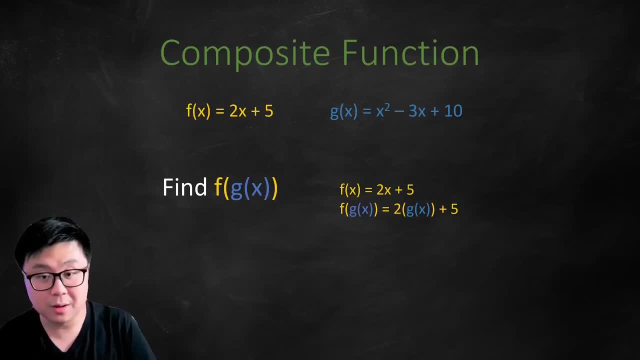 do that to both the left and the right. Now, on the right side, recall that g of x is actually x squared minus 3x plus 10.. That's the actual function output of g of x. so we can substitute that on the right. You don't have to do that to the left. The left is just there to show that. 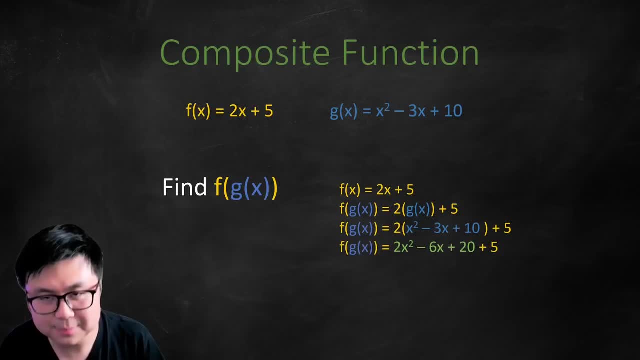 we're doing f of g, of x. Now on the right, you can continue to simplify And simplify until you get this composite function. One last note: this composite function, what they're asking for, can also be written in a different way, like this: f o, g, x, d, o is actually 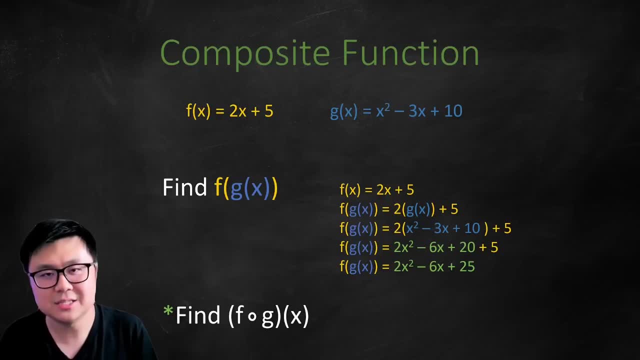 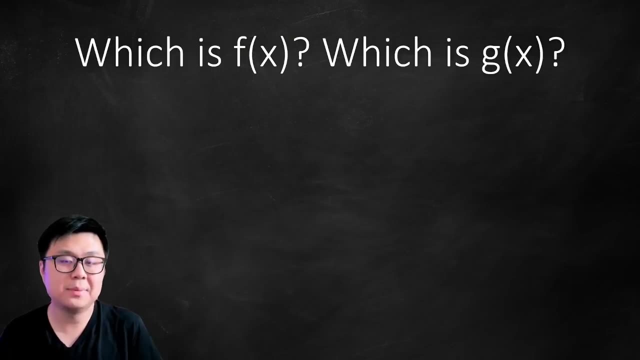 of. so it's f of g of x. That just means the second letter or the g is getting stuffed into the first letter or the f. Okay, so now you know what a composite function is, but unfortunately in calculus you actually have to look at a composite function. 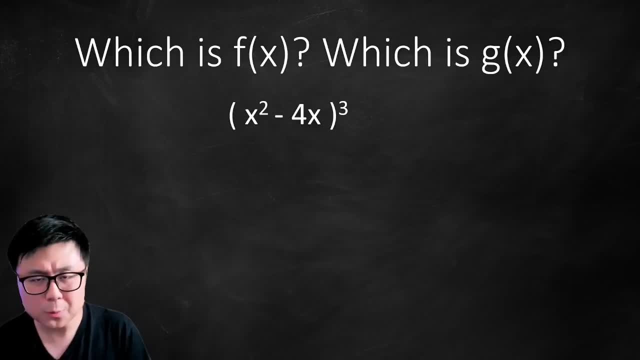 to be able to pull apart the f of x and the g of x. We have a bracket with x squared minus 4x inside, all to the power of 3.. Well, there's actually two functions in here. We can think of it this way. 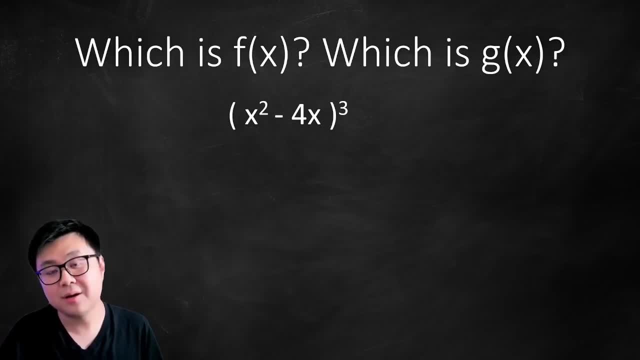 on the outside the brackets to the power of 3. could there have been just an original x in there And then we stuffed the x squared minus 4x into where the x used to be. so now it's inside the brackets. So in this case we have f of x. 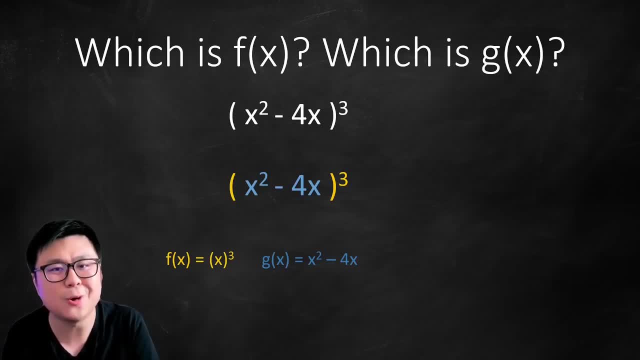 which is just x cubed. I'm putting brackets around the x to show that the brackets are there, and then the g of x, which is what we're stuffing into the f of x. and the g of x is x squared minus 4x. How do? 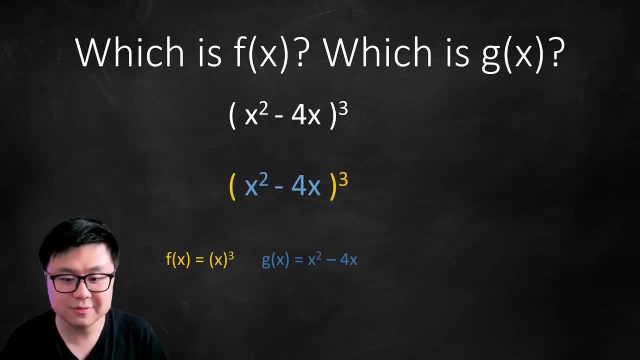 you know you're doing this right. Well, let's go backwards, right? If you were to stuff this x squared minus 4x into where the x is in the f of x, you would get that. Okay, let's try another one. log 2x cubed. Well, in this case, what stands out right away is the log, isn't it? Okay, well, 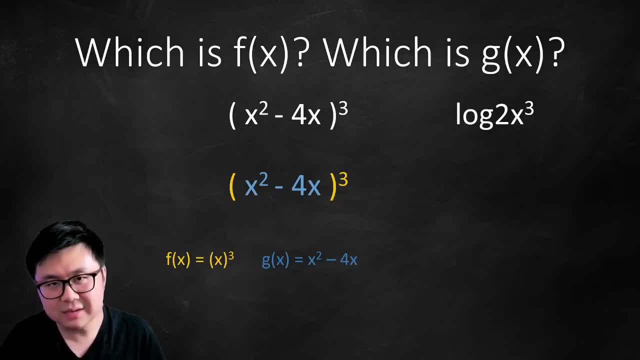 think what's the default function for a log. Well, the default function for logs is just log x. but I don't see log x. I see log 2x cubed. That means the 2x cubed is probably stuffed into where my x used. 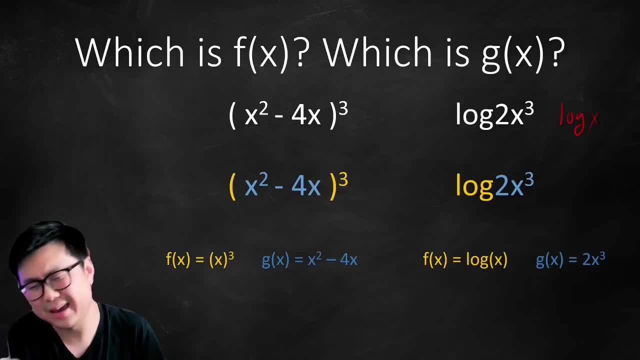 to be. so my f of x here should be my default log of x. Again, I'm putting brackets that show the stuffing here, and then the g of x is the 2x cubed and then, as you can see, if that goes into where the x is, we're going to end up with that. 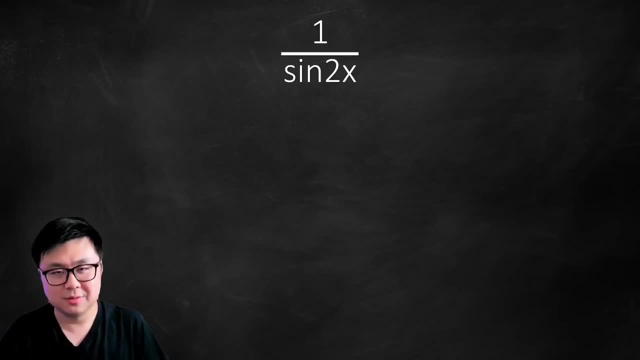 Now, the problem with this one is it's in a fraction, so the very first thing we have to do- we don't have a choice here- is to move the sine 2x to the top, although we get a negative exponent out of it, that's okay, not a big deal. Now, looking at this, does this look like a composite function? Yes, it. 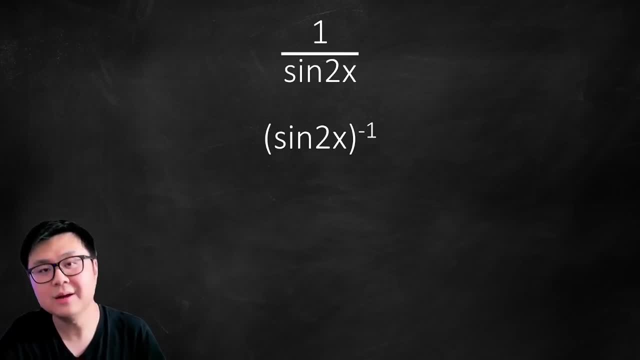 does, because why We have a bracket all to the power of negative 1? that's got to be my outer function. that's got to be my f of x. Well, what about the inside? The inside is sine 2x. Well, hold on a second. here the sine stands out. and what's the default function for a sine? The. 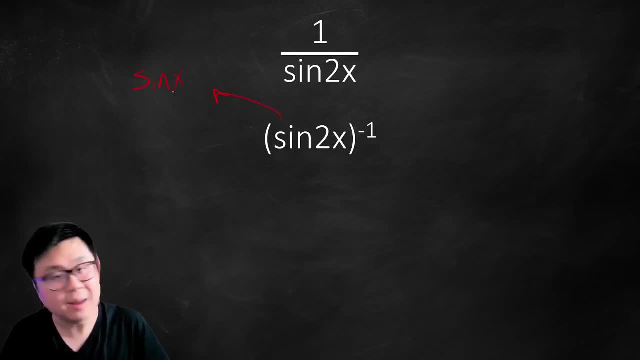 default function is just sine x, isn't it? But I don't see that. I see sine 2x. that means we have another function stuffed inside of my sine function, which is stuffed inside of my brackets, to the power of negative 1.. So, as you can see, we have a composite and a composite. the 2x is stuffed inside of my sine x. 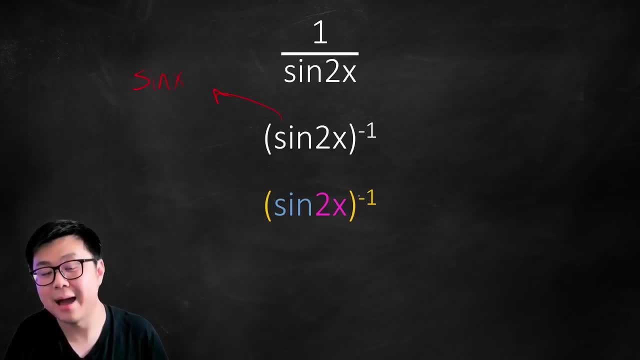 which is stuffed inside of my x to the power of negative 1.. Alright, last example of this video here, starting off with the problems here. what do we see? Well, we have a radical on the bottom. we don't like radicals in calculus, we like rational exponents. so let's write this as 2 over brackets. 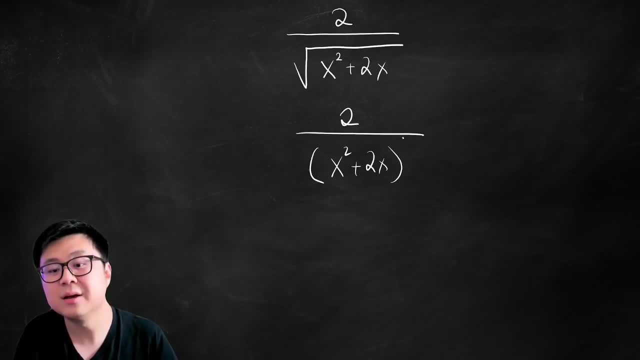 x squared plus 2x to the power of half. Okay, what's another problem? Another problem is we don't like fractions in calculus either. so we're going to move this bottom to the top, making it a negative exponent. but that's fine. So let's move it to the top and we're going to get 2 bracket x. 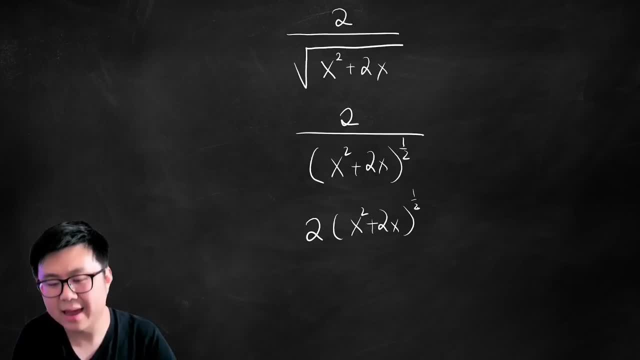 squared plus 2x to the power of a half. Okay, and at this point we can see that we have a outer function that is 2 and then a bracket to the power of half. so that can be my f of x here, My f of x. 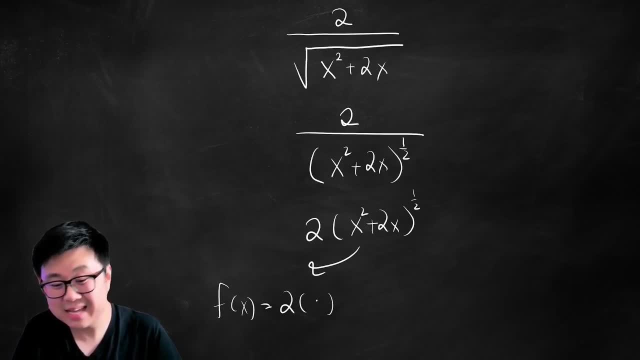 can be 2, and then that bracket should just have an x inside. keep it simple to the power of a half, and which means the stuff in the brackets that replaced the original x has to be my g of x. so the g of x should be x squared plus 2x. All right, we're done the video. finally, for those that made, 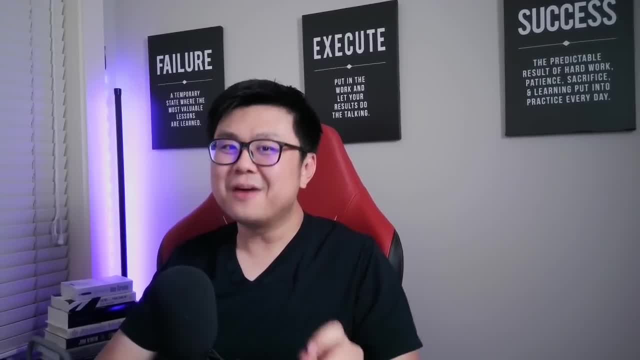 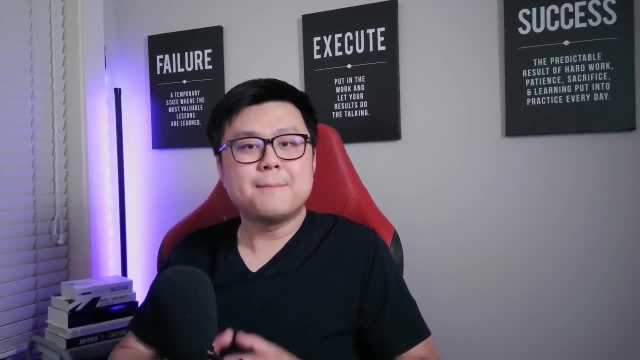 it to the end. awesome job and I can promise you it will pay off when you start calculus. Like I said, these five things we covered- they're not that difficult, they're actually pretty basic, but if you know them really well it will make your life in calculus so much easier. If you.